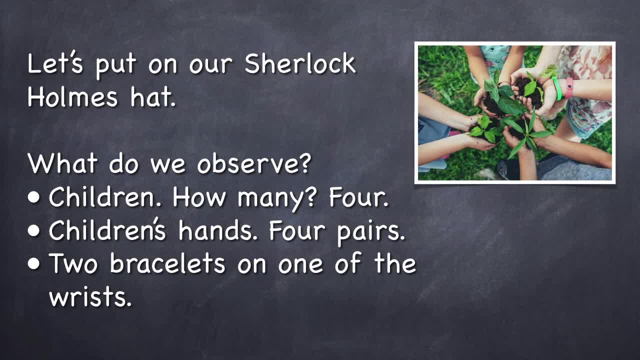 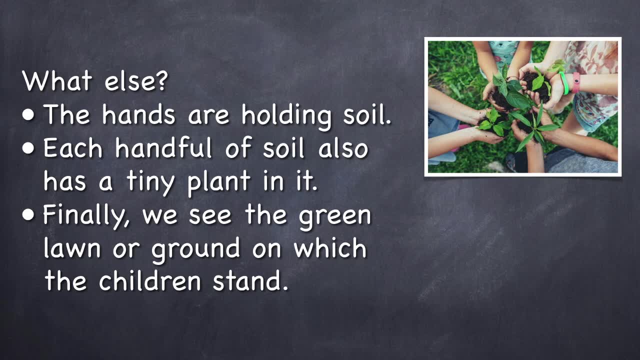 and these are just the basics. Okay, these are some of the human and some of the non-human elements. What else? We have the hands that are holding soil. right, They're holding soil. Now, each handful of soil also contains a tiny plant in it. And finally we see the green lawn or the ground. 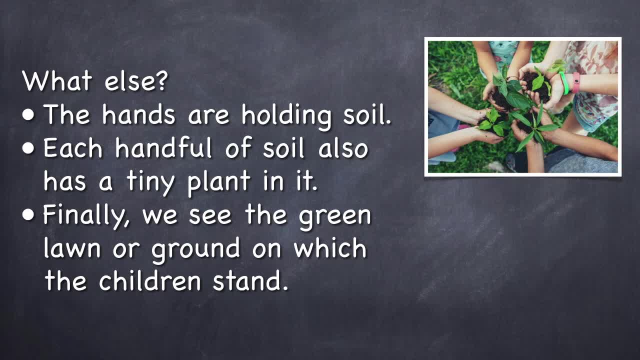 on which the children stand. In other words, we're identifying every single thing that we see in the image, so that it's not just a blur, it's not just a picture, It's no longer one picture, it's a bunch of elements, And we want to make sure we capture everything, Everything we can see. 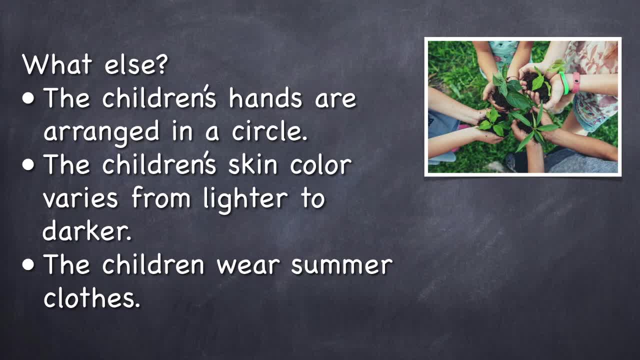 So what else do we observe? Now we observe, this would be the kind of the next level of paying attention to this. Okay, we're going a little bit deeper. So we notice that the children's hands are arranged in a circle. So we do see that. We also notice that the children's skin color 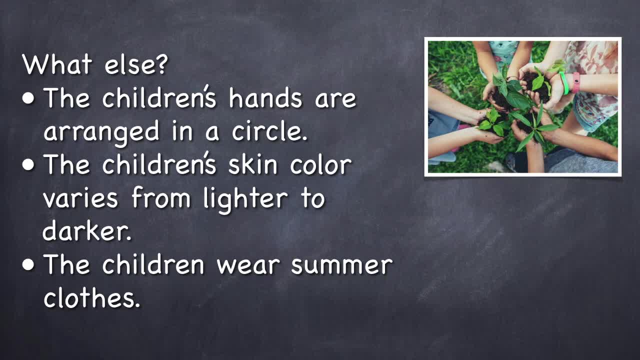 varies from lighter to darker. Some of them are a little bit darker, some of them a little bit lighter, And we notice that the children wear summer clothes. So that's another thing we notice. This is not the winter, clearly, right, This is the winter. So we notice that the children wear. 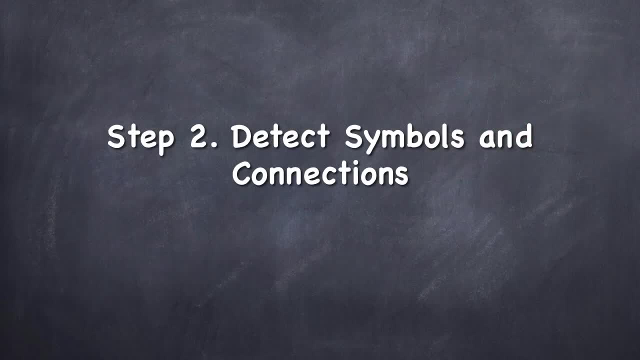 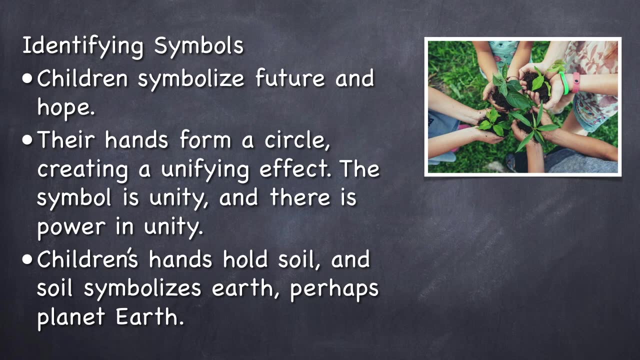 summer. Okay, next. Next, we're going to detect symbols and connections. In other words, we're going to be interpreting some of the things that we have observed already. We're making some interpretations here, So let's identify some of the symbols Now. children symbolize future, and 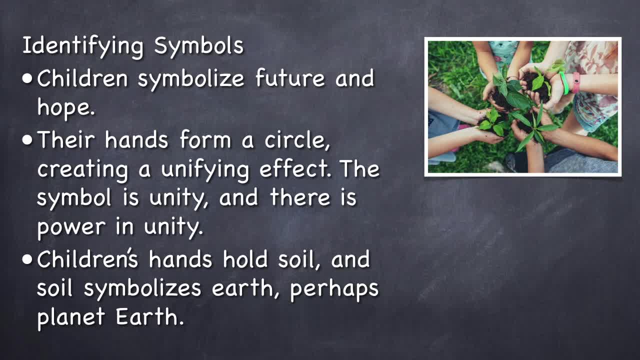 hope, right, Because they are children. Next, their hands form a circle, creating a unifying effect. Now, a circle kind of unifies, right, The symbol is unity And there's, you know, a lot of power in unity. See, we're already deriving some meaning from the elements. 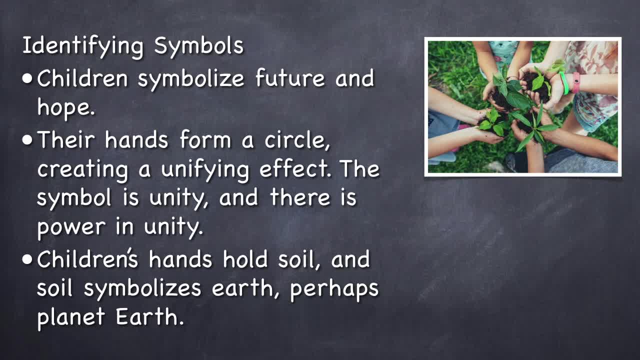 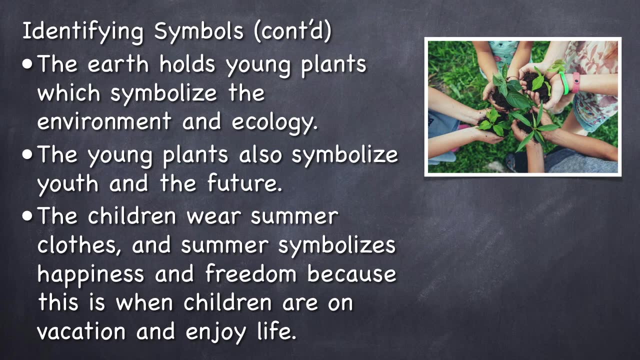 Next, children's hands hold soil, and soil symbolizes earth, perhaps planet earth, In other words. note that another word for soil is earth. So we're going to continue. The earth holds young plants, which symbolize the environment and ecology. Okay, that's another symbol. Now 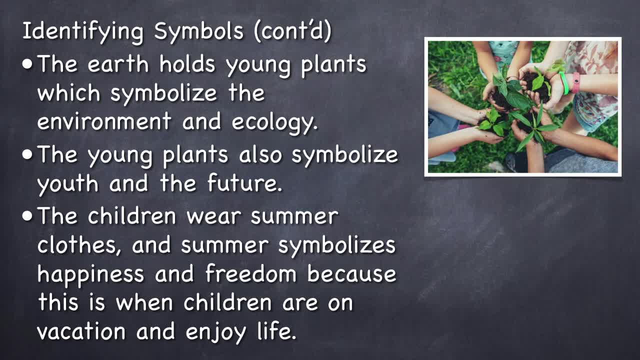 the young plants also symbolize youth and the future, Because notice that, you know, the human beings in this image are young And also the plants in this image are young. Both are kind of, both symbolize childhood and kind of the future. Next, the children wear: 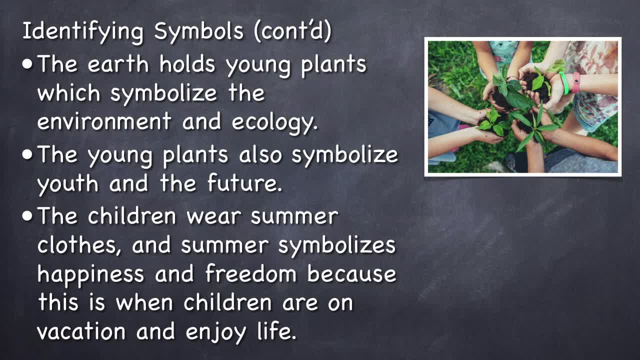 summer clothes, And summer symbolizes what It symbolizes: happiness and freedom, because this is when children are on vacation and enjoy life. So there's no school right, So there's freedom, kind of happiness and the kind of joy of life, that type of thing. So we're. 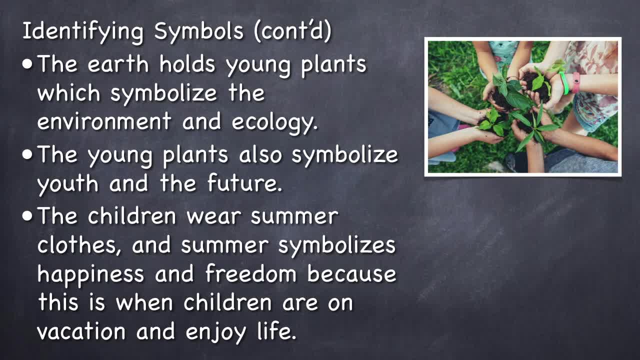 inferring all of the stuff from this image. You see, these are some of the things that we need to do, And we're not even writing anything, We're just jotting down the notes. We're just, we're just noticing things and taking notes. Now let's find some connections and relationships between. 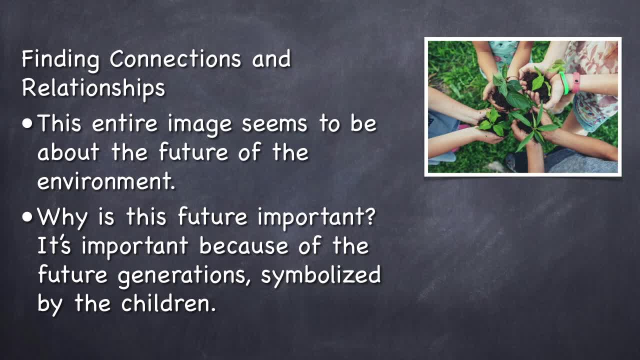 the elements and some of the symbols that we've seen. This entire image seems to be about the future of the environment. How do we know that? Because of all the things that we have inferred right, The children symbolize the future, The plants symbolize the future and the environment. Now, why is this future important? 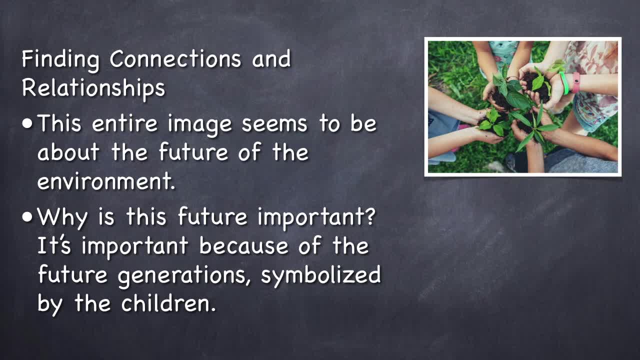 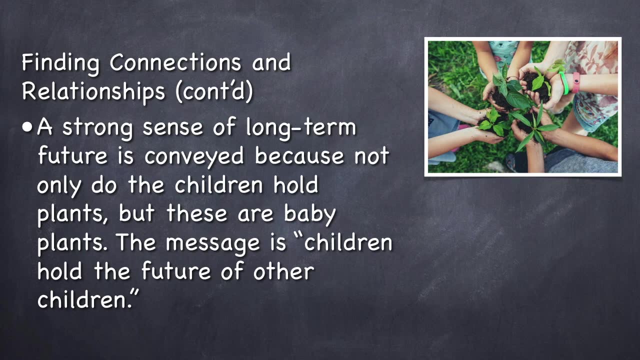 It's important because of the future generations symbolized by the children. You see, we can infer that, We can infer all of that from just by looking at this image more closely. Now we're going to continue. Now there's a strong sense, a strong sense of long-term future is conveyed. 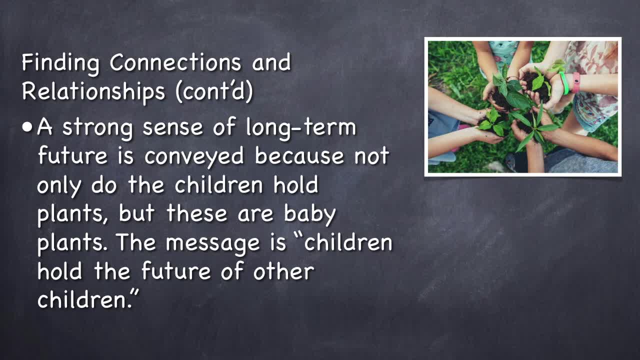 because not only do the children hold plants, but these are baby plants, right? These are also young plants, And the message here is that the future of the environment is going to be the future of the environment, And the message is, or could be, that children hold the future. 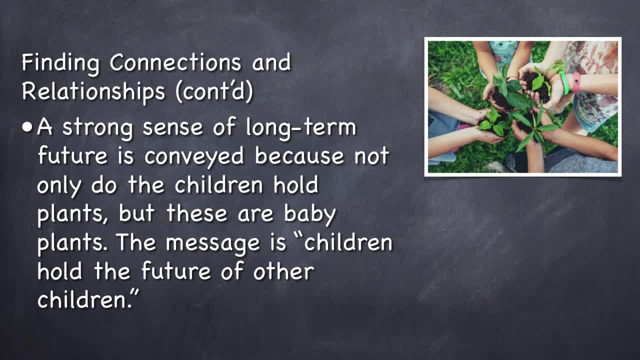 of other children. okay, It's a bit of a repetition, It's a bit of a tautology, but don't worry about it, We're just taking notes, We're just thinking aloud, and we're taking notes And we're going to. 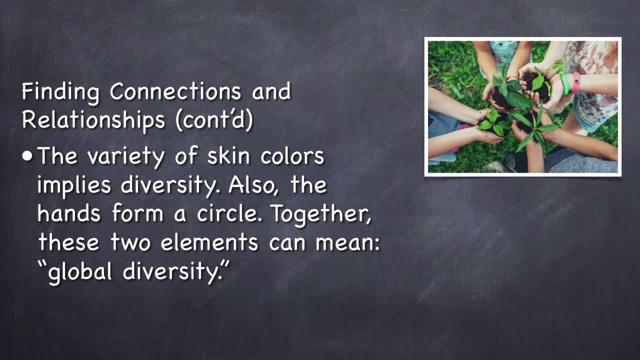 use that as we're writing out our essay. Let's continue. The variety of skin colors implies diversity. There we go. That's another thing. So also the hands form a circle. So together these two elements can mean global diversity. Why global? Because of the circle. Why diversity Because of different skin. 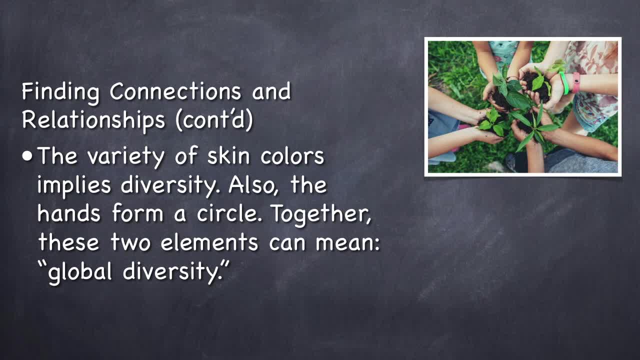 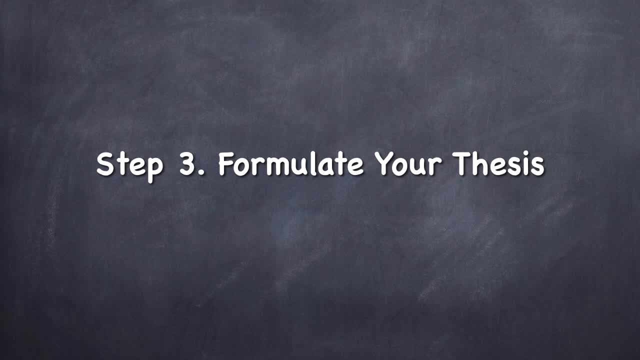 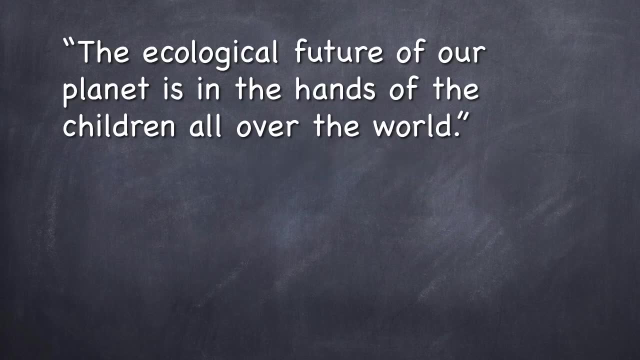 colors, right, Global diversity. There we go. We can definitely infer that from the image. Now that we have identified all the elements and the relationships among them, and all the symbols, now we're ready to formulate our thesis, And our thesis could be the ecological future of our 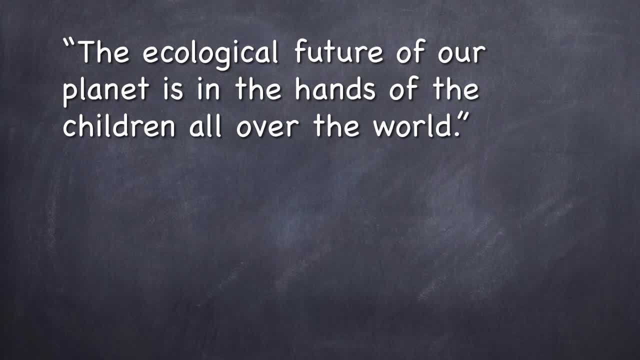 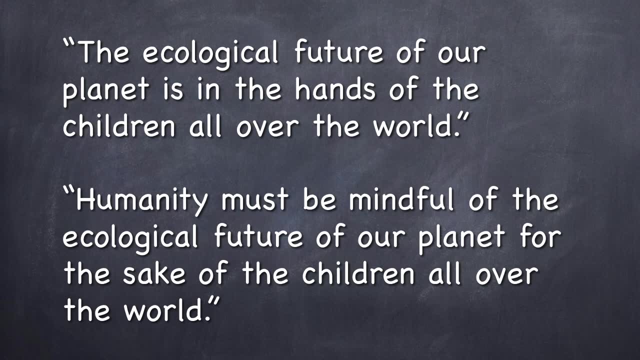 planet is in the hands of the children all over the world. This is one interpretation. Here's another one: Humanity must be mindful of the ecological future of our planet for the sake of the children all over the world. And these are two different statements. Now let's see which. 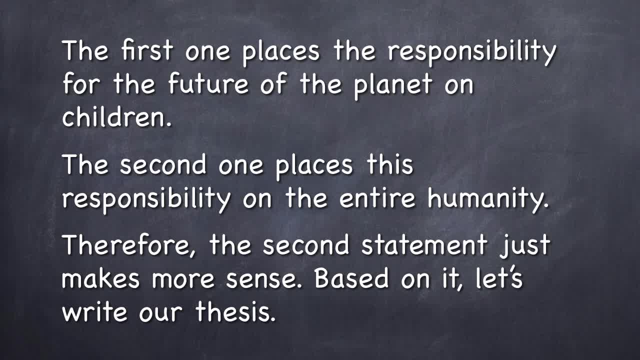 one could work a little better, I think. well, the first one places the responsibility for the future of the planet on children. Okay, Now the second one places this responsibility on the entire humanity. Now, which one makes more sense Now to me? I think that, therefore, the second statement. 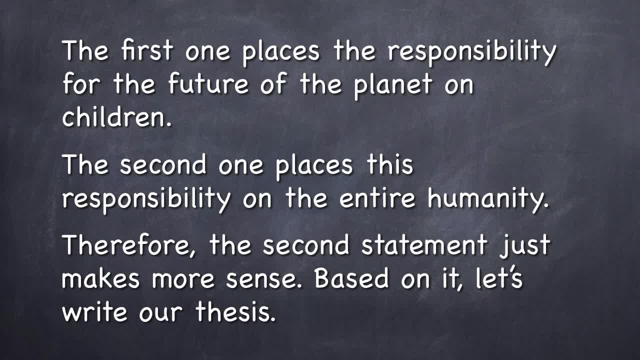 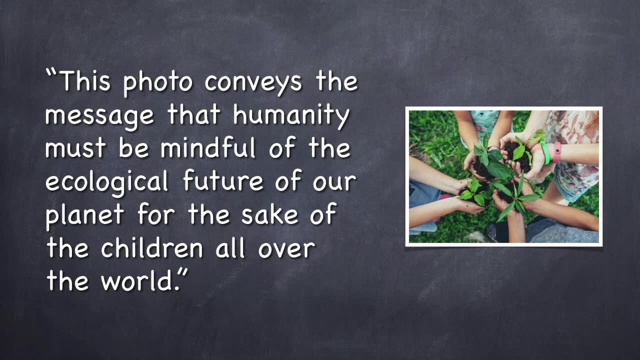 just makes more sense. Why? Because we're putting the responsibility on the entire humanity rather than on kids. Okay, So based on that, because it's more logical, let's write out the thesis Now. this photo conveys the message that humanity must be mindful of the ecological future of our 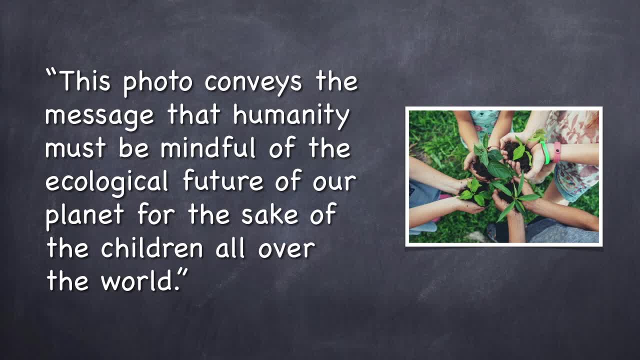 planet for the sake of the children all over the world. You see how we came up with this main point: based on the elements that we identified. Just by identifying all the elements, or the symbols, and connections and relationships among them, and taking notes, we can put together a thesis just like this one. Okay, And formulate it Why? Because now we have. 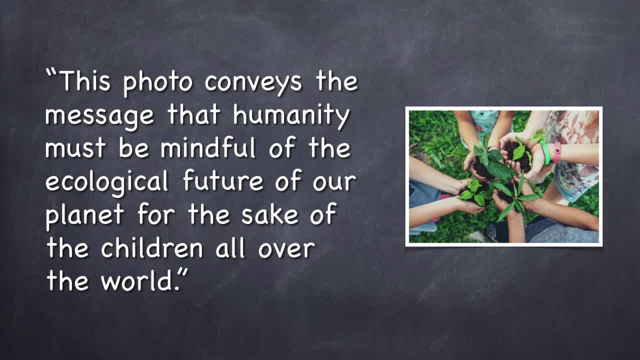 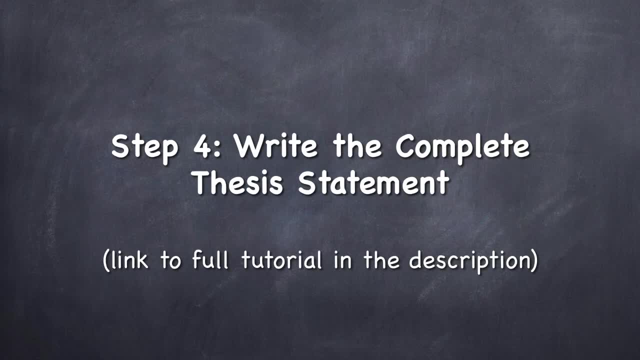 the building material to formulate a complete thought, a complete main point, And let's say that this is the complete main point that we're making in this essay. Now let's write out the complete thesis statement, And I do have a full tutorial on the subject and I'm going to include 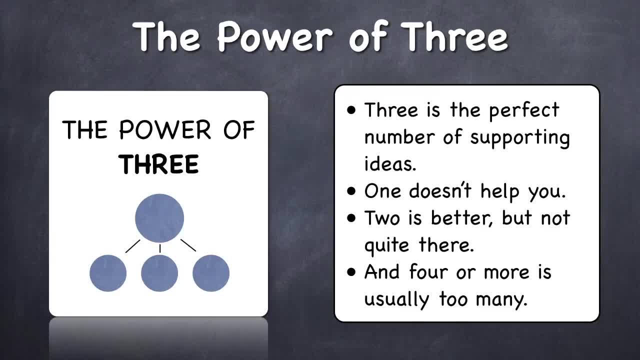 the link in the description And we're going to use the PowerPoint, So let's go ahead and write out the full PowerPoint. Now, if we agree that the picture has value, it goes into the output and we're going to create three pieces that are hostile to the parallel. This is our view of the picture. 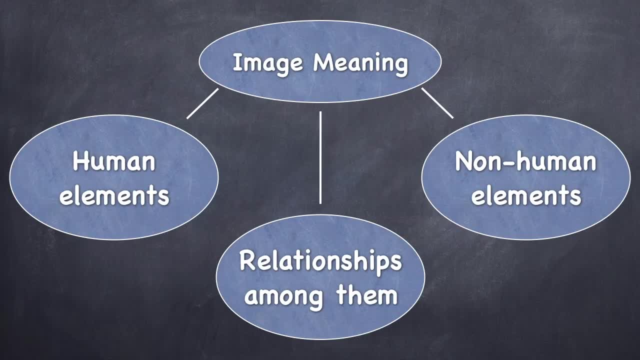 Lets make a few corrections on power and if we want to be honest with you or something, Okay, So in this slide we have this Pizza fim. I see these series as conforming ohne fashion. What I'm actually seeing here is that this picture is Tactics. just to see that. 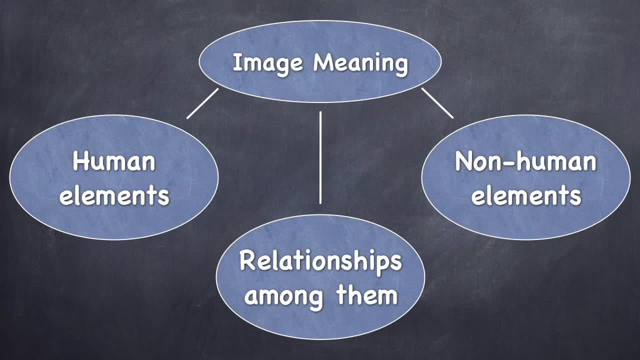 this has value and how you can actually relate to something else, a thing like schonking into you arms and things like that. What is it going to contribute? Can you show them how they've actually contributed the very same thing weplay to, For example, the stage art, and I don't really know? 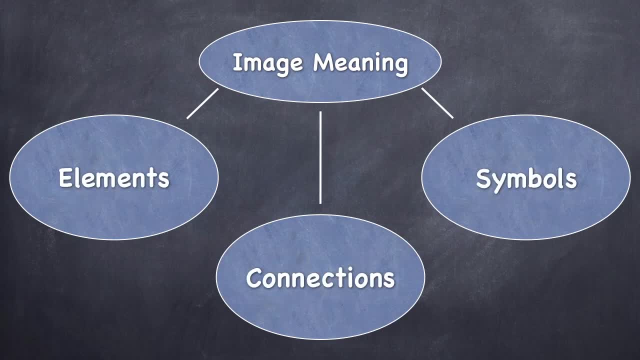 because this guy said that he's kicking people up a bunch and he might as well just jump his clothes. here's another way of doing it we could have. we could talk about the elements, we could talk about symbols and then we could discuss the connections among them. that's another way of doing it, but it's also the power of three. 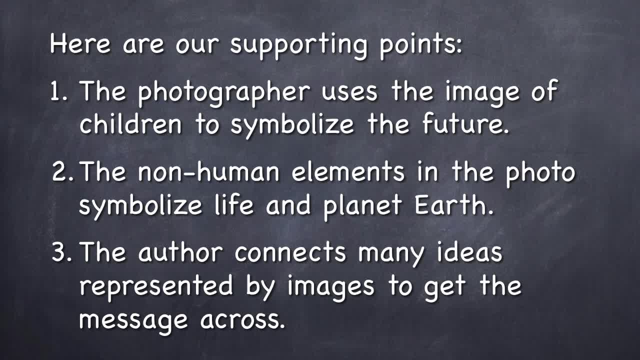 all right, so here are supporting points, and let this let's decide on these. number one: the photographer uses the image of children to symbolize the future. okay, we already know that from the work that we've done previously, so this is just the one that we're using here. 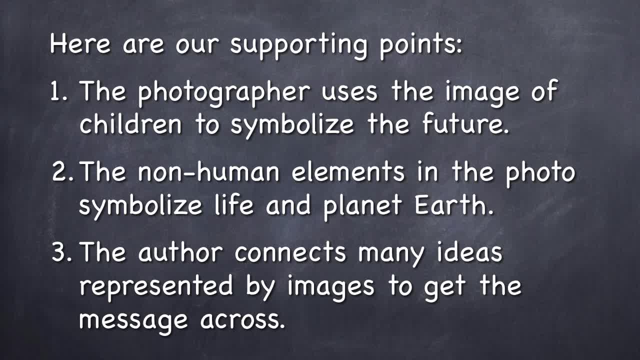 next, the non-human elements in the photo symbolize life and planet earth. okay, the soil, the circle, the, the little baby plants. these are the non-human elements. and next, the author connects many ideas represented by images to get the message across. okay, let's write out the complete thesis. 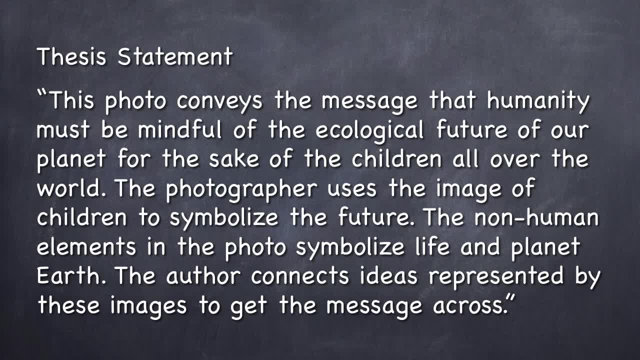 statement, and we have everything we need to to do that. so here's the complete thesis statement. okay, let's write out the complete thesis statement. okay, let's write out the complete thesis statement. this photo conveys the message that humanity must be mindful of the ecological future of our planet for the sake of the 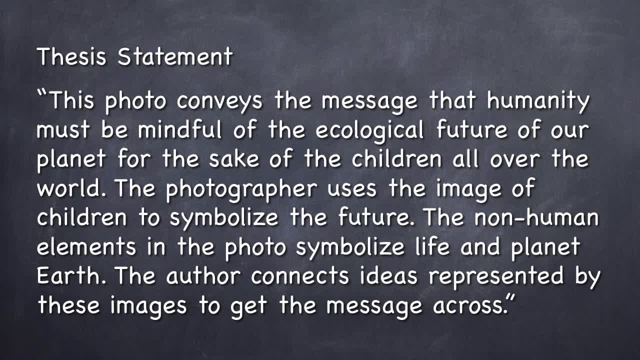 children all over the world. the photographer uses the image of children to symbolize the future. the non-human elements in the photo symbolize life and planet earth. the author connects ideas represented by these images to get the message across. you see, and that's a complete thesis. 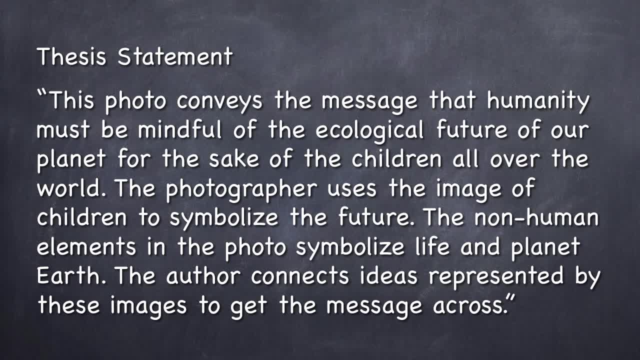 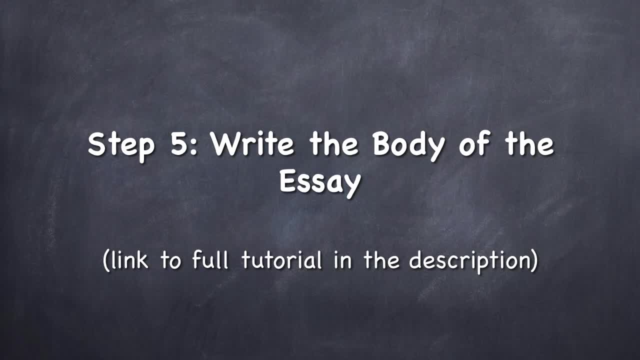 statement because it has the main point and it has all the three supporting points and we also have a full paragraph. going in step five we're going to write out the body of the essay and i also have a full tutorial on how to write body paragraphs and i'll include 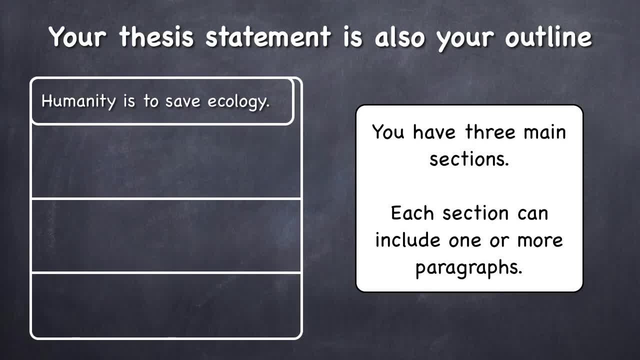 the link in the description. now, remember, your thesis statement is also your outline, so we already know our main point is: humanity must save the ecology. okay, that's that's pretty much our main point. now we have three main sections. how come? because we have three supporting points: human elements. 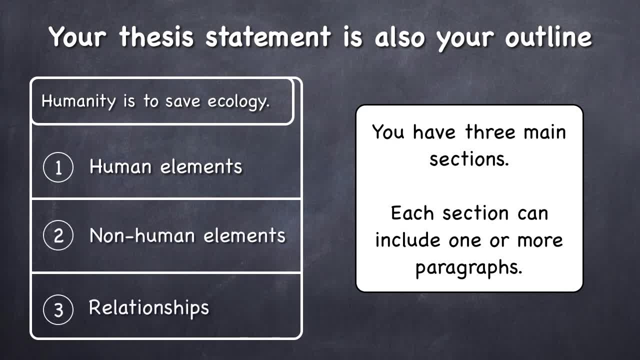 non-human elements and relationships among them. we have three sections. each of them can include one or more paragraphs. so don't think in terms of paragraphs, necessarily think in terms of sections, and a section could be one paragraph or more. now here's our body paragraph structure: a body paragraph. 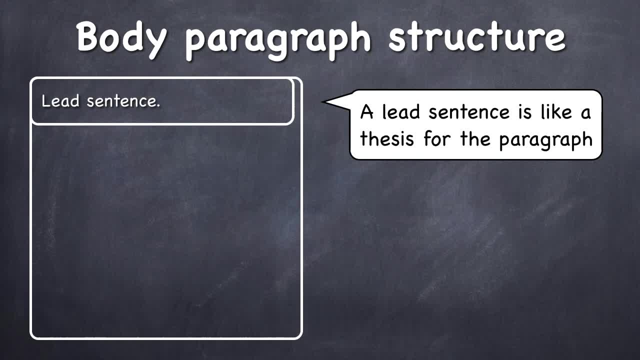 begins with a lead sentence and it's like a thesis for the paragraph. it's the most general statement. next we have an explanation, right between one and three sentences- you will usually do- and finally we have examples, also between one and two, maybe three examples, but one if. 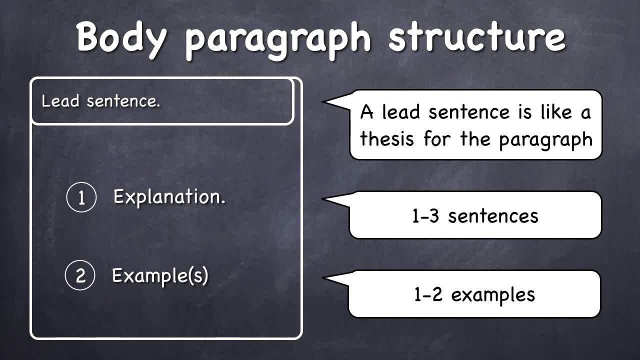 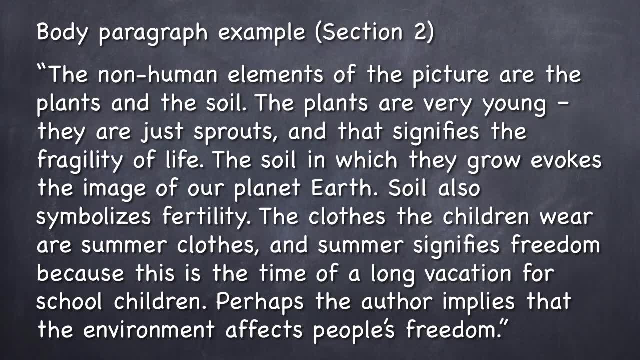 one will do. two is better, three maybe, depending on how many words you really need in this essay. okay, and that's our body paragraph, anatomy. and let's do an example of a body paragraph and let's take one from section two, where we're talking about the non-human elements. the non-human elements of the picture are: 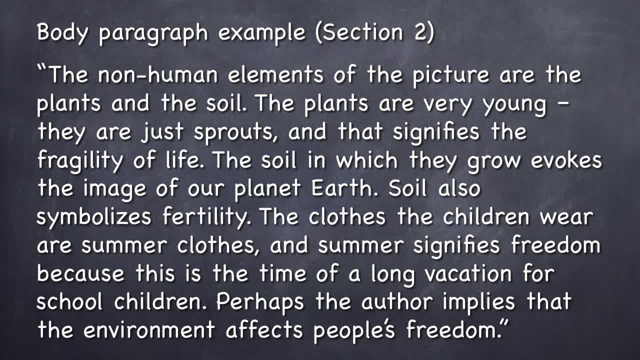 the plants and the soil. the plants are very young, they're just sprouts, and that signifies the fragility of life. the soil in which they grow evokes the image of our planet earth, and the plants are very young, they're just sprouts, and that signifies the fragility of life. the soil in which they grow evokes the image of 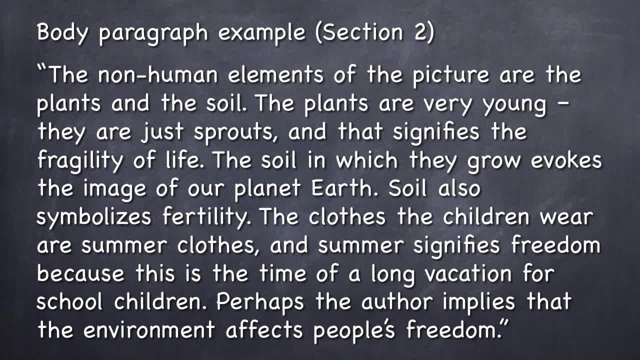 soil also symbolizes fertility. the clothes that children wear are summer clothes, and summer signifies freedom, because this is the time of a long vacation for school children. perhaps the author implies that the environment affects people's freedom. all you really doing here is you are using the new. 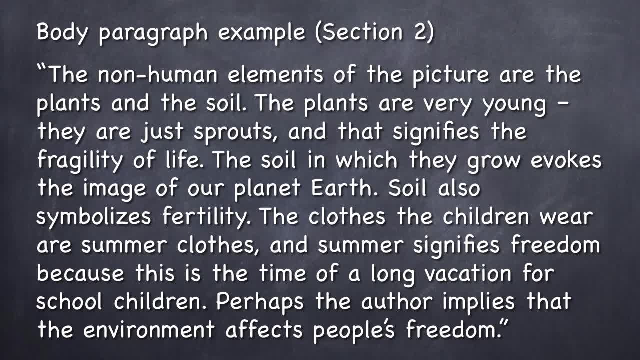 using the information from the notes that you took when you were analyzing the, the image, when you were taking down the notes about all the elements of the symbols and all the relationships between the person and the environment, that you, the relationships among them And you're, you're constructing a. 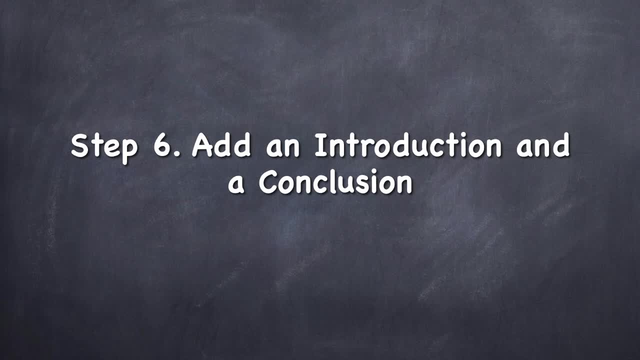 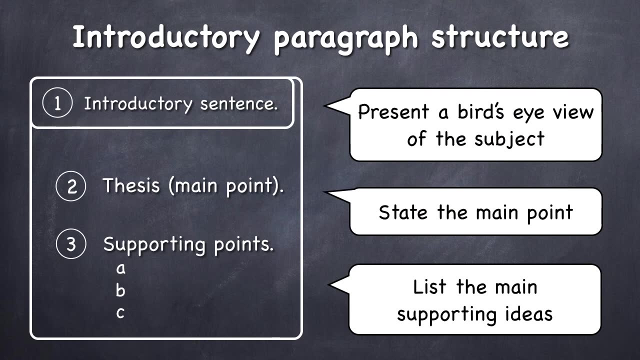 complete paragraph, going from general to specific. Finally, in step six, we add an introduction and a conclusion. Here's the structure of an introductory paragraph. we begin it with an introductory sentence, then we present the thesis and then the supporting points. Now we already have our main point, And 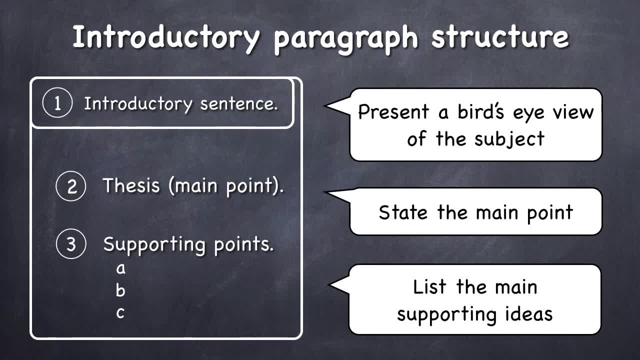 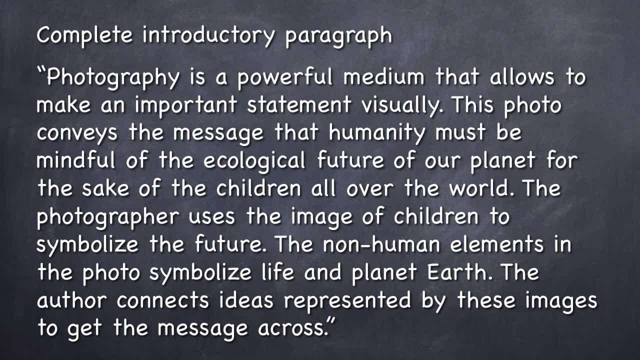 we already have our supporting points, So we already have parts two and three. Now all we need to do is add an introductory sentence. So here's our complete introductory paragraph, And notice that the first sentence is the introductory sentence we just added. Photography is a powerful medium that allows to 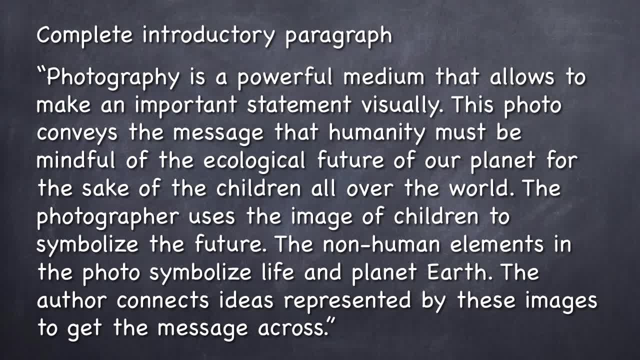 make an important statement. visually, we're making another very general statement, And we're now going straight into the main point. This photo conveys the message that humanity must be mindful of the ecological future of our planet for the sake of the children all over the world. There's our main.